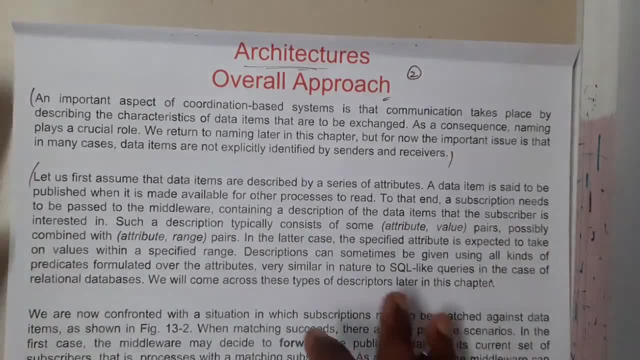 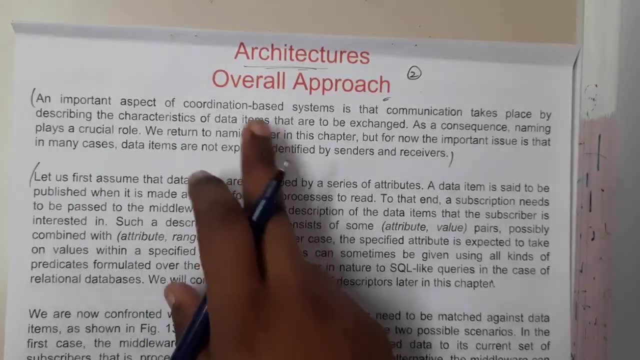 are really easy. You can remember them and you can write in your own words, guys. So first let us go through some kind of basic theory. After that we will be moving on to the diagrams. So an important aspect of coordination based systems is that communication takes place by describing. 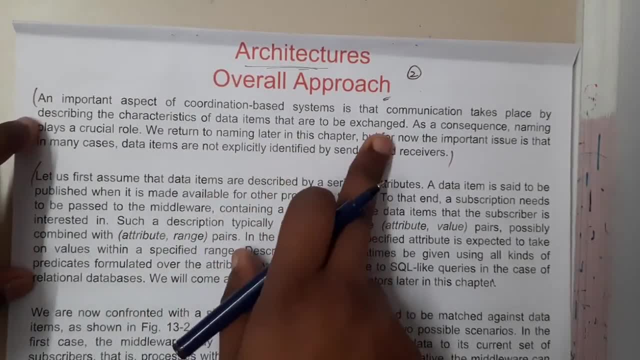 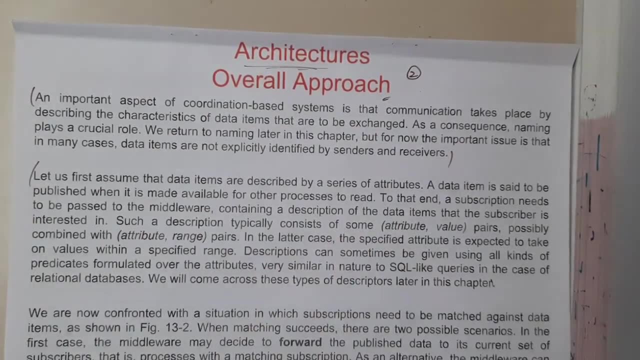 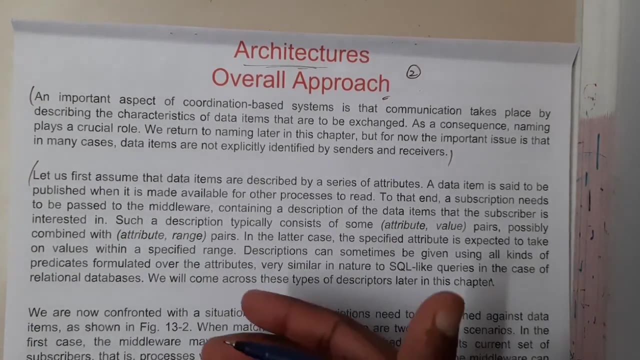 the characteristics of data items that are to be exchanged. as a consequence, naming plays a crucial role here. So basically, assume that you want to buy a book, guys. So assume that you want to buy the book of distributed system only. So if you want to buy the book, you need to know the book. 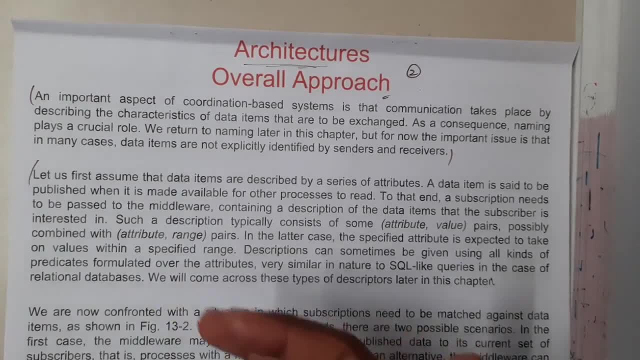 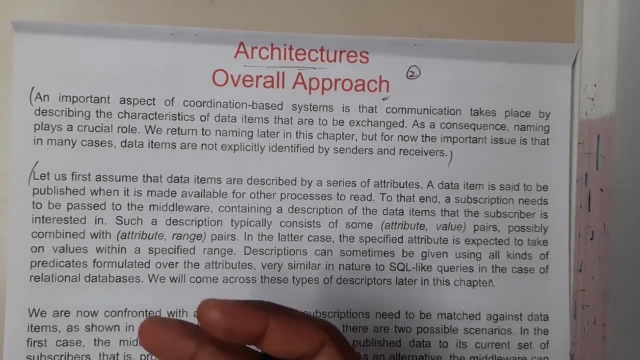 name Along with the author name, right? So you cannot go to a shop and say the distributed system gave me the book, So he will be giving four or five books. He'll be showing. if it's a big showroom or big shop, you'll be getting multiple books, right? Yes, So if you say distributed systems, 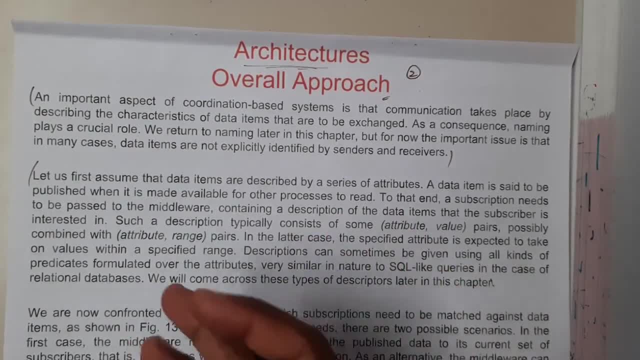 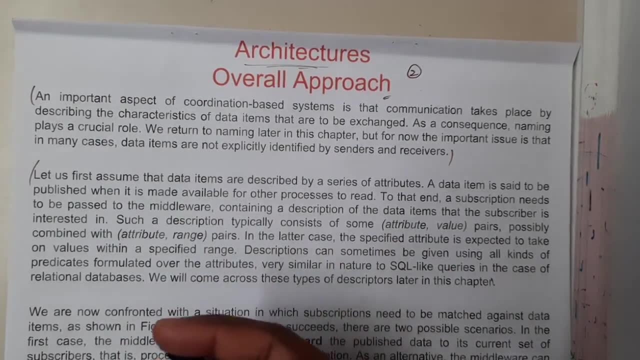 of a principles and paradigms. so in that situation you will be getting the exact book which you want, right? Yes, So in that way you should know the name, the identity. only then you can get the things easily, right? Yes, So that is the same concept which we'll be using in this. 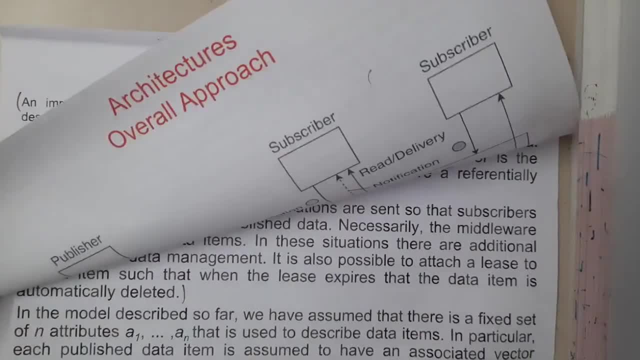 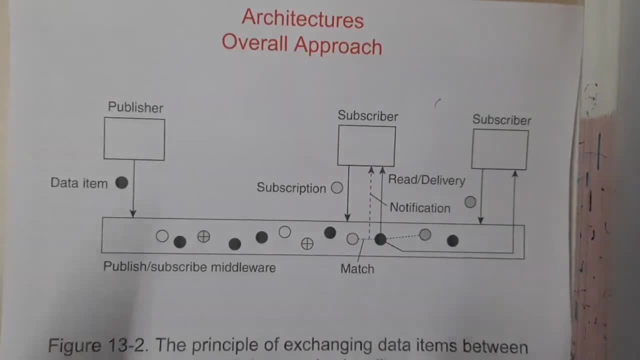 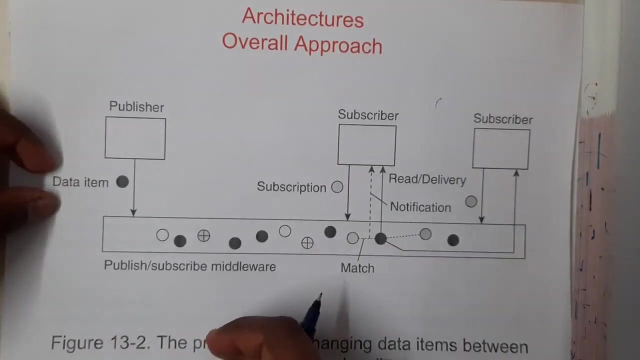 coordination systems also. Okay, Yes, Okay. So let us go through the first diagram. This is nothing but just the exchange of data. guys, We'll be discussing the detailed subscribers and publishers a diagram, Don't worry So this is just an introduction diagram. You can say: okay, Yes, So basically the publisher will be publishing his 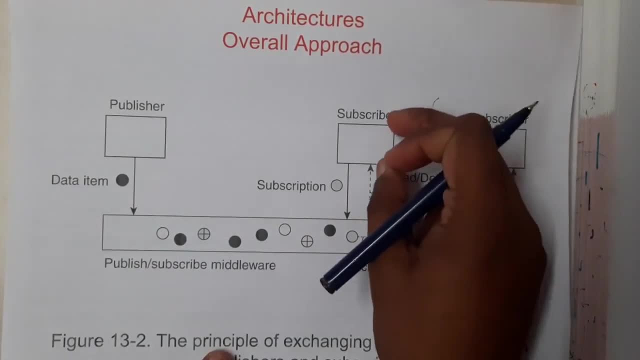 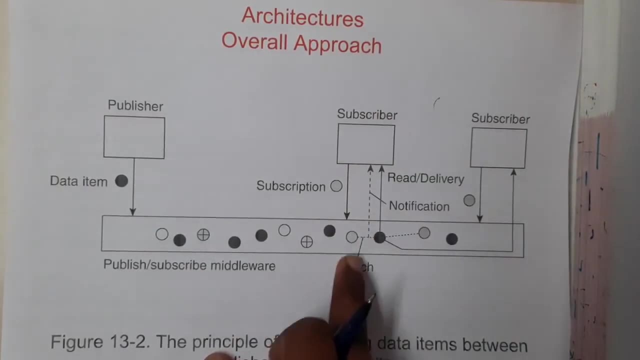 data into the channel, guys, Okay, And based on the subscriber requirement, based on those names, the tags and all those things he'll be, he'll be sharing his data. That is nothing but his requirements He'll be sharing. So if he's a data and our data he's a request, assume that. 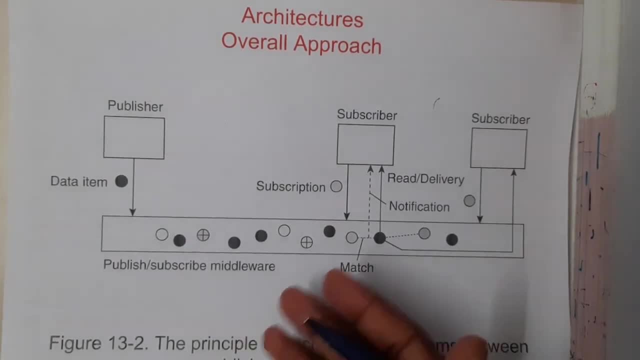 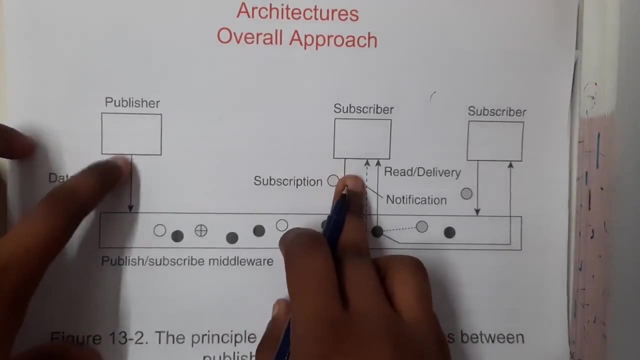 he's searching for some video on coordination based systems. Okay, Architecture diagram. Okay, So he typed on YouTube. Okay, So he typed and I also published. at the same time I published the same video. Okay, So he searched and it is also published. So these two will match right, Yes, So. 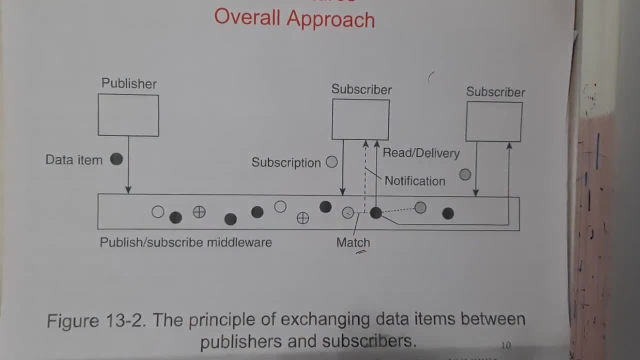 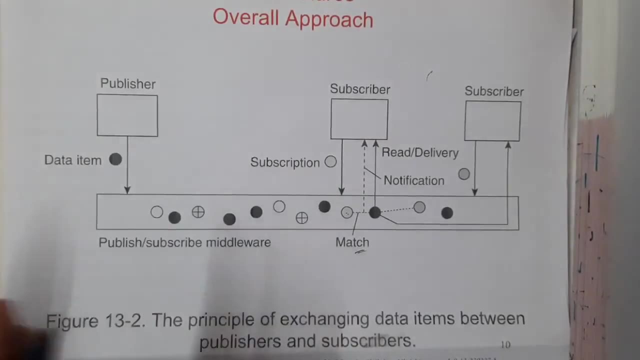 these two will match and the video will be coming in his search result. So in that way. so this is the model, guys, of subscribers. So basically we can have multiple subscribers, but for a particular channel or particular thing we can say only one publisher will be there, right? Yes, There will be. 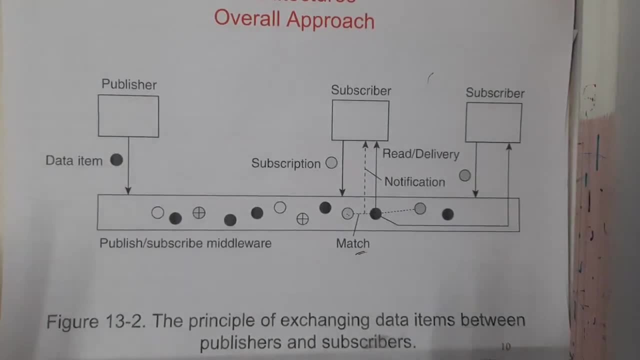 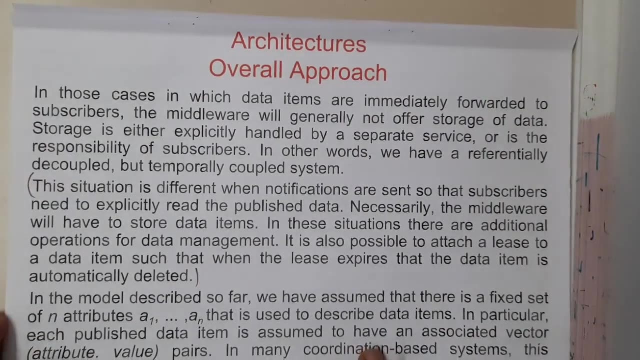 multiple actors, but only one owner of the channel will be there, right, It's under one only email ID. I mean, right, Yes, Okay. So this is the basic diagram, guys, Okay, Yes, Okay. So, basically, who is going to take care of all those videos? guys, the middleware. 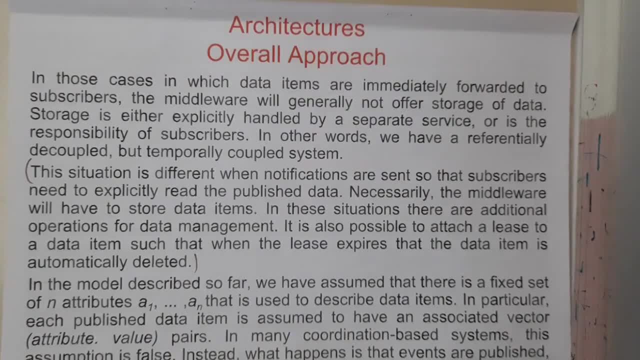 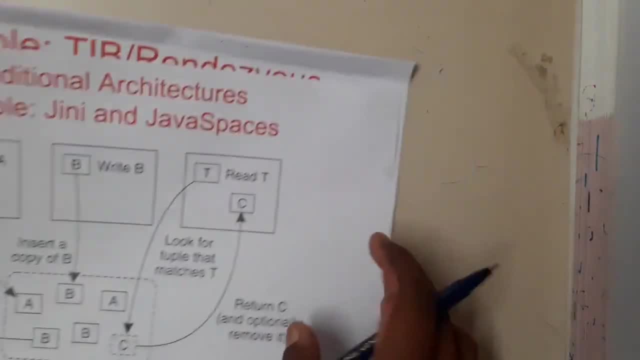 the middleware will be pushing those videos, storing those videos and all those things, right, Yes, Okay, So you can go to the theory. guys, It's really the same things which I was saying are written in the book also, So you can just go through them, Okay, So one of the traditional 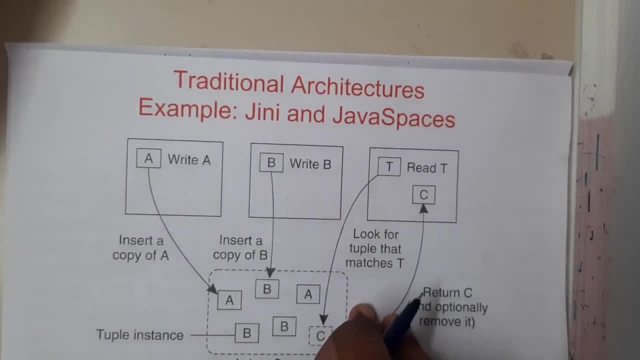 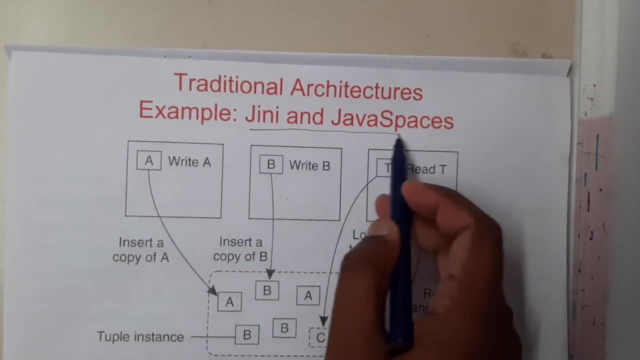 architecture for this coordination based system is, I told you, right? So your coordination means one or something will be done, right? Yes, So one of the popular is a tinny and Java spaces guys. Okay, So assume that there are three different processes and they need to do some operations. 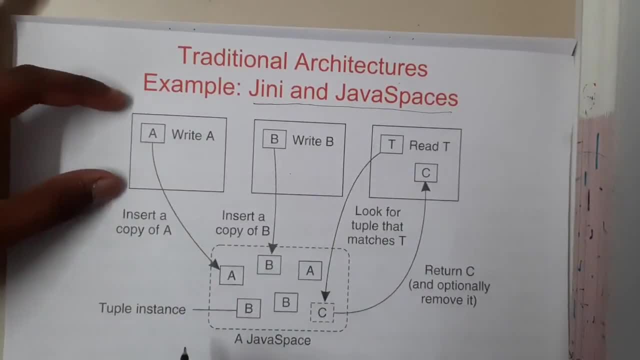 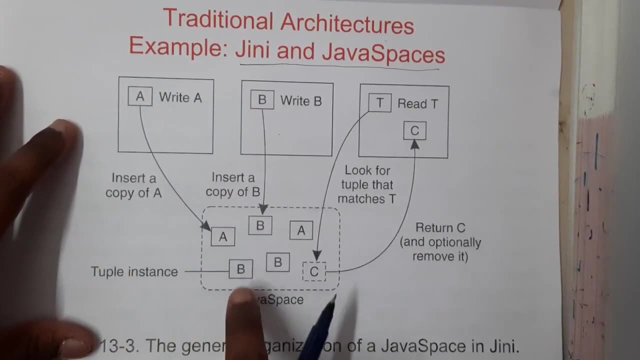 Okay. So in that situation, assume that you wrote a process, first process and second process are writing some values to your Java space. So we are writing A and B here, Okay, And already there are some tuples. assume in that way, guys, Already these three tuples are existing in the in our Java. 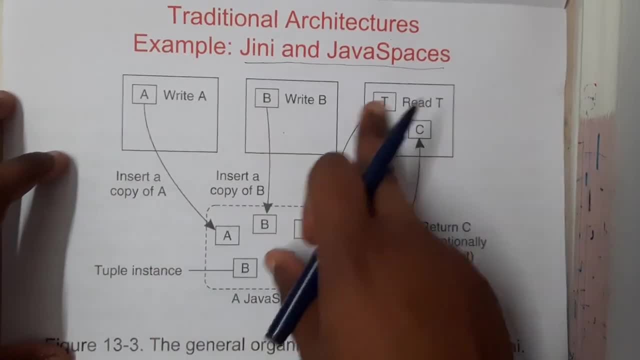 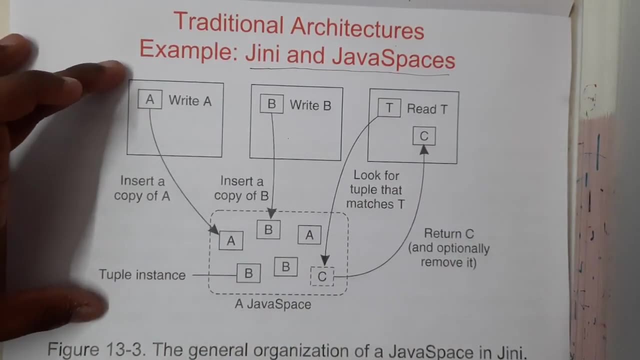 space. Okay, So once you enter the new tuples and if someone comes to read any kind of tuple, if it is existing or not, that will be read the guys and any kind of operation could be done. So if you observe this carefully, this also looks like the publisher system, right Publisher and subscriber. 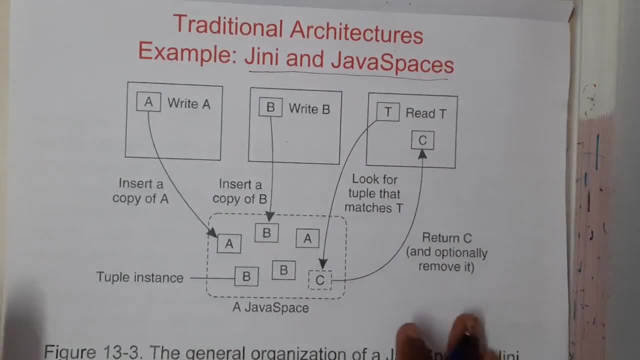 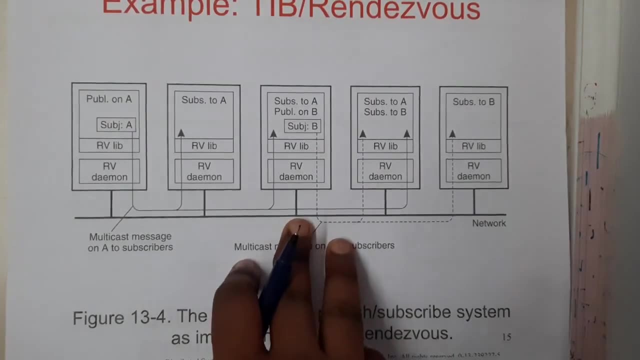 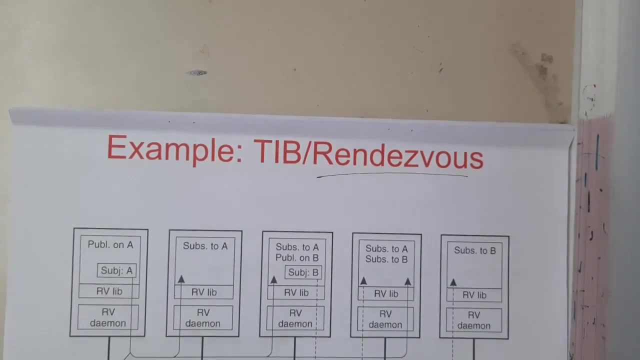 system, But the only thing is here, we can have multiple publishers. That's it right? Yes, So this is just a simple idea that I gave you guys. Okay, So I hope everyone got some basic idea on this. Okay, So now let us go through Tim, or? okay, You can just pronounce it guys. Okay, Yes, So this is. 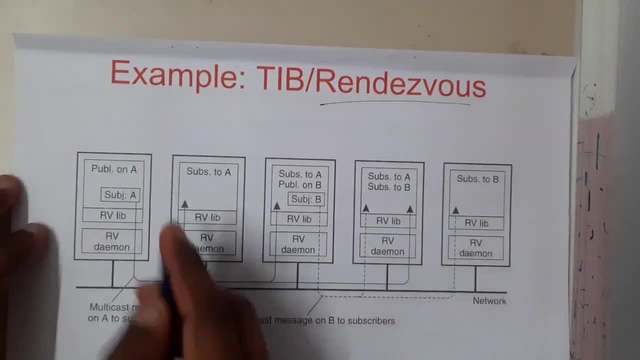 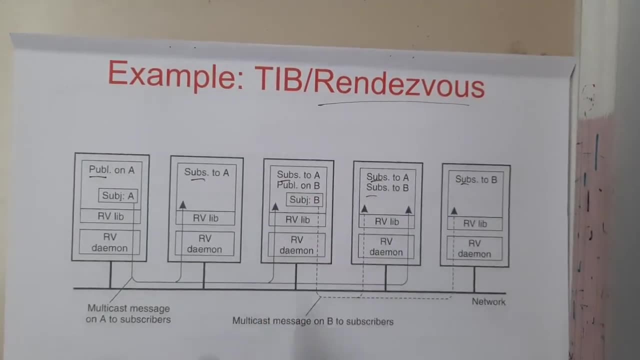 also a subscriber, publisher- Uh, diagram, only guys. So if you observe here, here we are having one publisher and many subscribers, guys, right, Yes, So even some subscribers could be publishers also, right? So even I subscribe for some channels and I also produce the content in that way, right, Yes So? 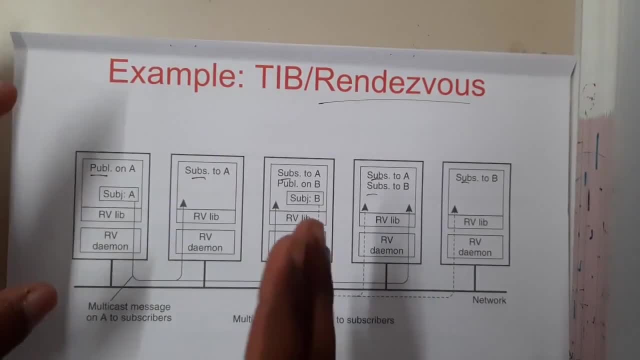 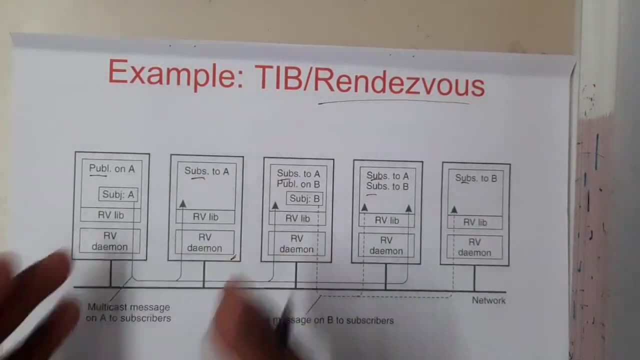 publishers. so publishers will be publishing the data, but you should remember one thing is the one thing which the subscribers will be using is nothing but RV domain guys. So that is the thing of which is stores everything Like. whatever you are searching, the request, everything will be. 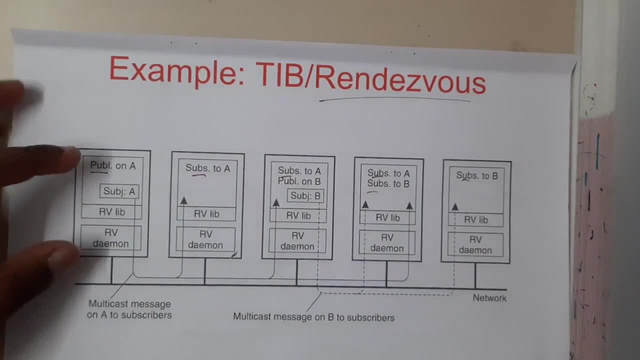 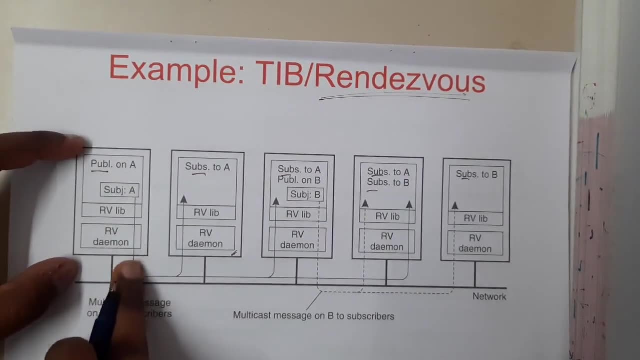 passing through it guys. Okay, Yes, Okay. So RV is nothing but this guy's, Okay, Yes. So basically the whenever the publisher publishes. so based on the request from the subscriber- previously I told, based on the request. So 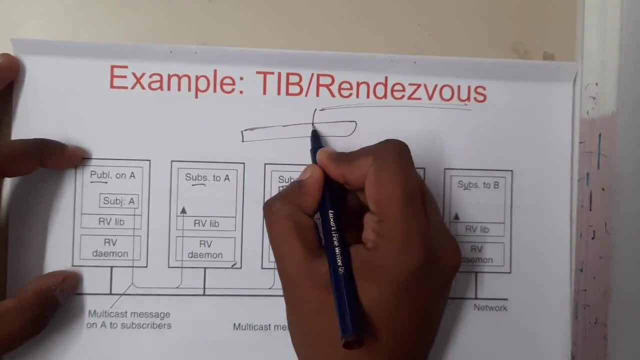 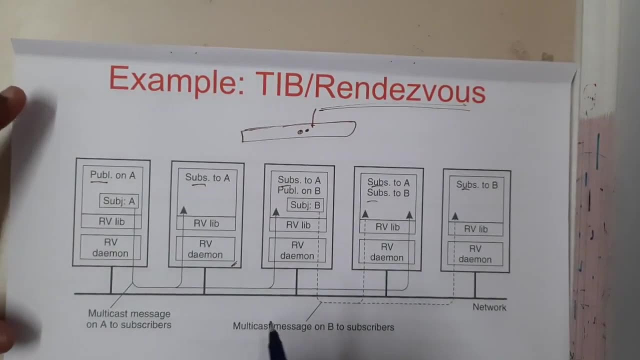 basically, it is already existing in that list And whenever a subscriber comes, he will be checking whether it's matching with his. if he matching, he'll be taking right. So that is our previous system, But nowadays, if you observe, even in YouTube, if you upload a video automatically, 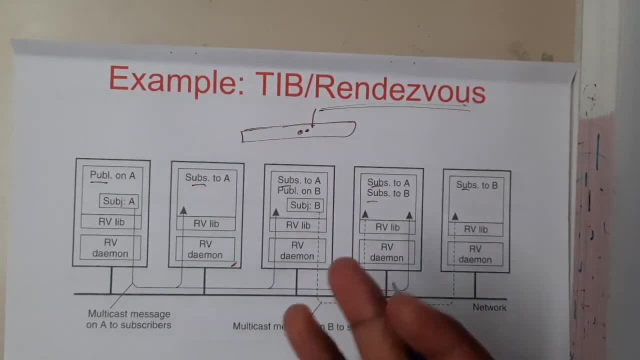 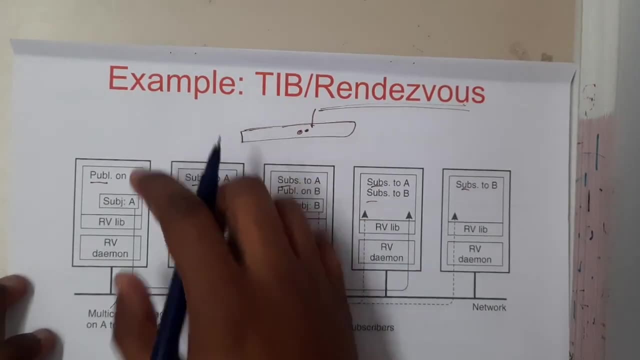 most of the subscribers. if they turned on their bell notification, they'll be getting a notification that your favorite YouTuber has uploaded the video Like. then you'll be able to getting right. Yes, So in the same way, this will work, guys. So basically, here you will be only. 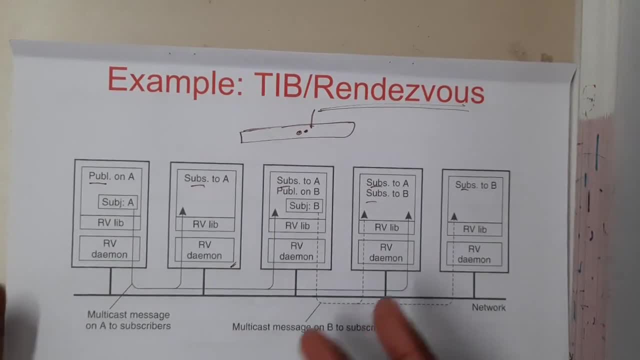 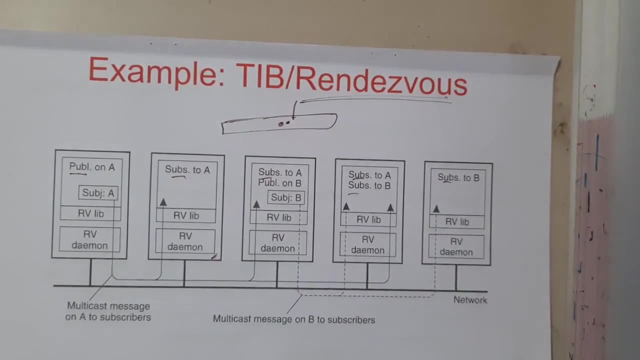 sending the, sending the message to everyone based on your requirements. So basically, if you don't want to send to this guy, you will not be connecting with this. So if you notice here, the last subscriber did not got the notification because he didn't click the bell icon, like that. 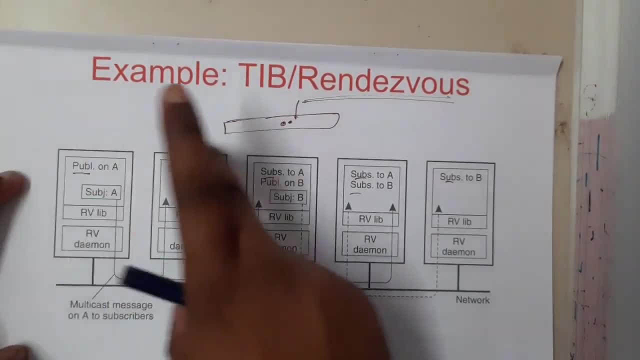 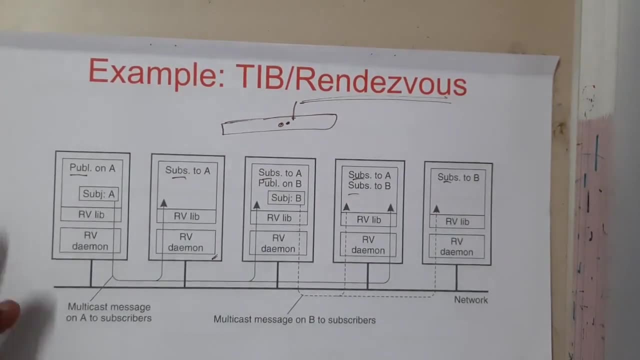 So I am just giving you an example. Okay, Yes, So that concept, the exact concept, is nothing but this T I B or ran ran Zobo's diagram. Okay, Yes, So this is the principle that they are going to use. 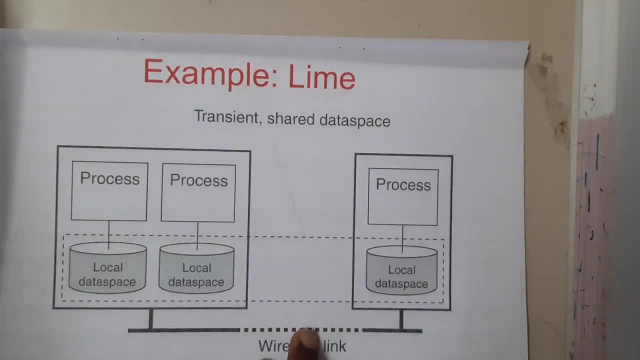 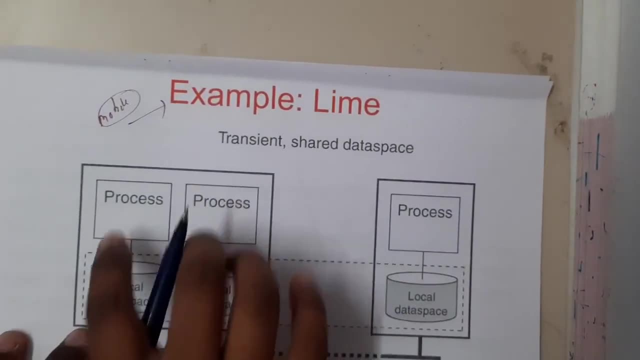 Okay, Yes, Okay. So let us continue. So this is used in mobile guys. So whenever you are using your mobile device- this is the backend, like each and every process- will be communicating with the local databases guys. So basically, they will be using your own phone databases, right, Okay So? 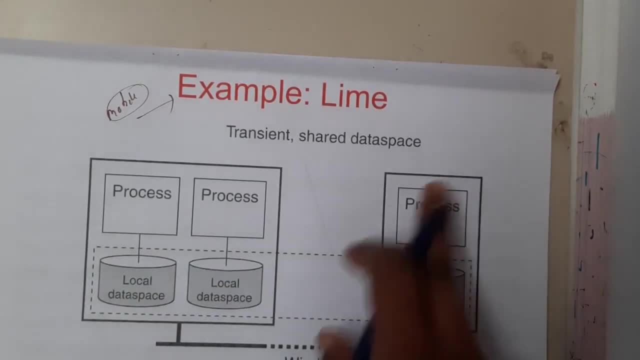 based on that. if I need a request, is there any kind of data? they'll be moving onto the internet, They'll be getting the data from that particular site or somewhere and they'll be showing it to you in that way, Right, Yes, So this might not be that much related, but it is given in the 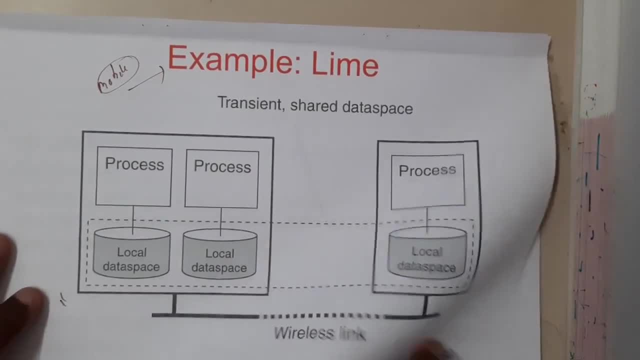 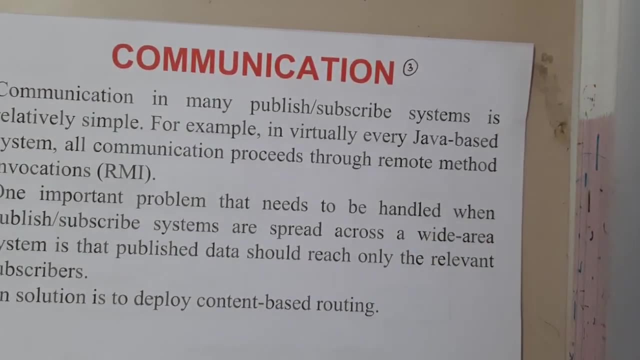 PPT and even in the textbook also. Okay, So that's the reason why I'm explaining it to you. Okay, Yes, So I hope everyone got some basic idea about some architectures. So in the next lecture I'll be discussing about the communication guys, So how communication can be done in this. 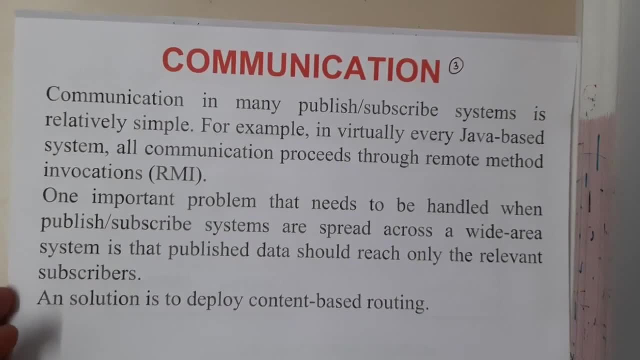 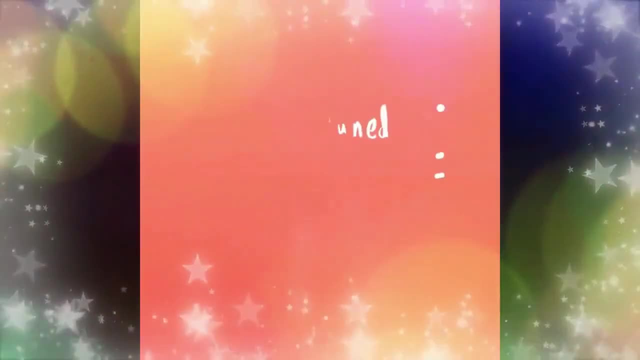 coordination system. Okay, So let us meet in the next lecture, Thank you. Thanks for watching.